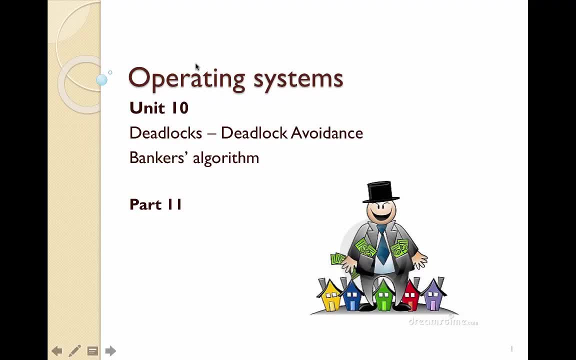 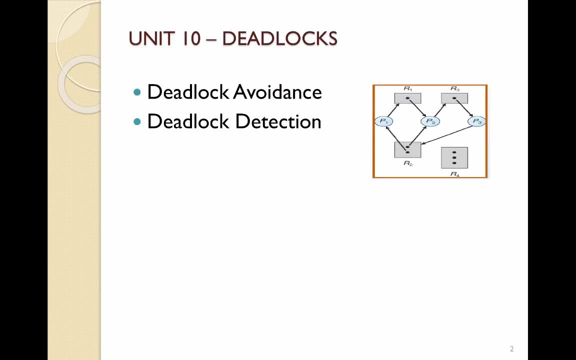 Welcome to operating systems. unit 10, part 2 on deadlocks, deadlock avoidance and the bankers algorithm On deadlock avoidance. processes use resources and they share different instances of different resources, and processes need to indicate which resources they need and the operating system needs to make choices on how to allocate the resources to the process. 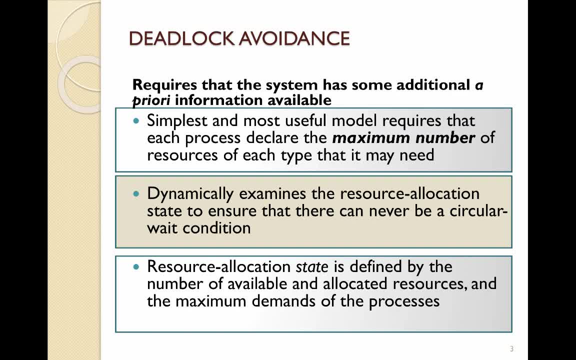 and keep it in a safe state. So the simplest way is for each process to indicate the maximum number of each resource that it needs, and then the system will allocate these resources in a way that when a process finishes using that resource, it can be freed up and used. 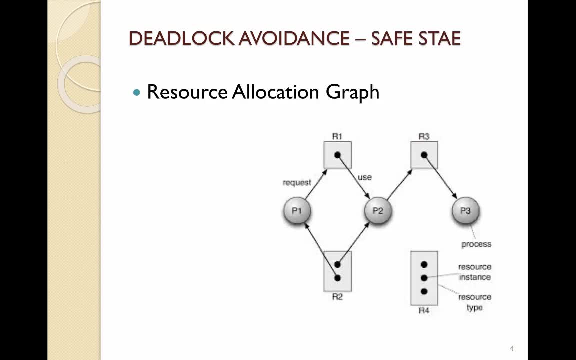 by another process. So one way to do this when you have limited numbers of the resources is just to use a resource allocation tool. This is an allocation graph where processes make a request for a resource and resources are allocated to processes And in this situation we have three processes: P1,, P2, and P3, and 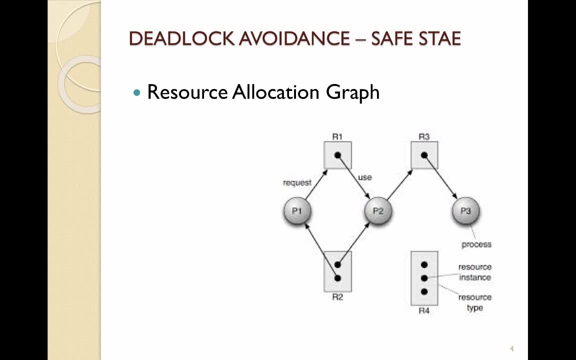 we have four resources: Resource 1,, resource 2,, resource 3, and resource 4.. And the dots in the resources indicate how many instances there are of each resource. So, as you can see, P1 is requesting resource 1 and there's only one instance of it and it's in use by. 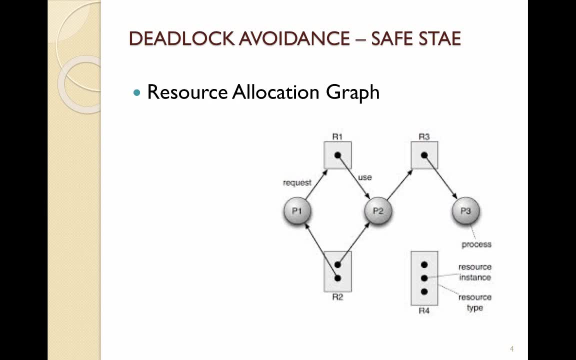 P2. Which is also using resource 2, but it's also requesting resource 3.. And resource 3 has been given to process 3.. But you can see that there won't be any problem here, because when process 3 is finished with resource 3, it will be free, and then P2 can use resource 3, resource. 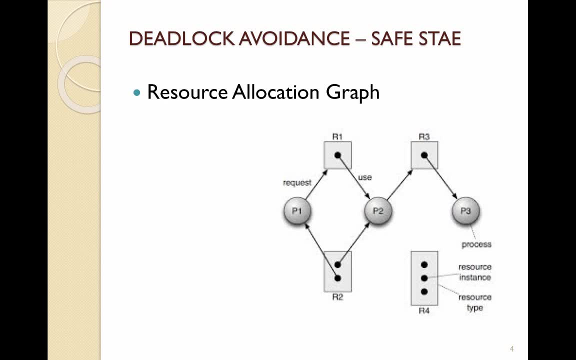 1, and resource 2 and free those up, and then P1 can use resource 1.. So we have a safe situation here. If P3 were to make this request, which were P3 is requesting resource 2, then we have a problem because we have cycles in the graph, and when there is a cycle in the graph, then 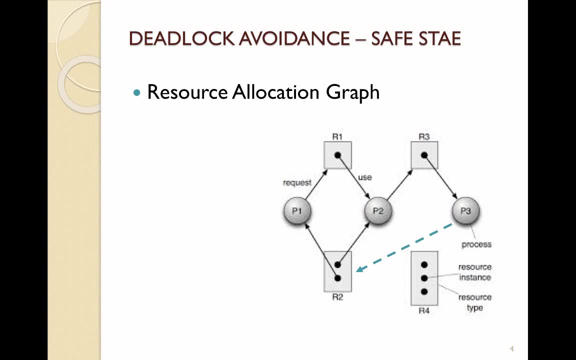 there's. there's a chance you will have a deadlock, because if P3 makes the request for resource 2, there's no way for P3 to free up resource 3- for I mean for P2- and we have a deadlock situation. So we have two cycles here: One cycle that starts at P1 and ends 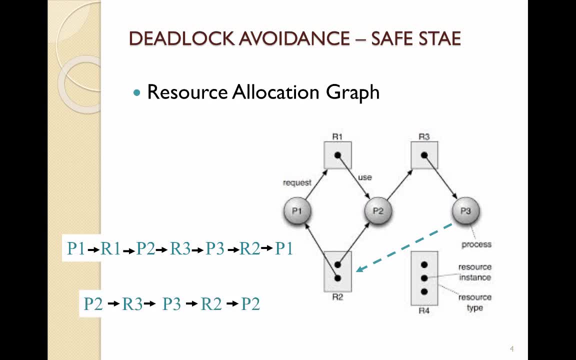 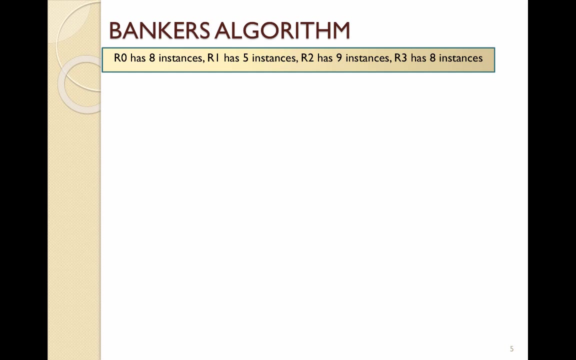 at P1, and a second cycle that starts at P2 and ends at P2.. So when you have a cycle, then you are not, then the system is not in a safe state. Now we're on to the Banker's Algorithm, which is a way to allocate multiple instances. 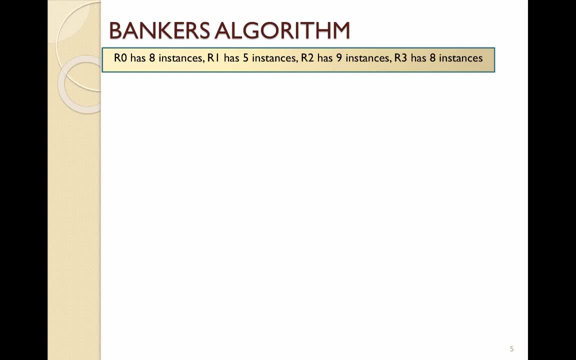 of resources. So if there are, in this case we have four resources: 0,, 1,, 2, and 3, and there's eight instances of resource 0,, five instances of resource 1,, nine instances of resource 2,. 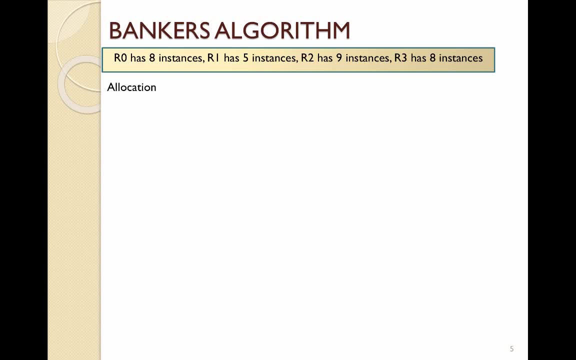 and eight instances of resource 3.. So the Banker's Algorithm. what happens is we have a couple of matrix here. we have each process, we have five processes and these five processes are using these different resources. So what happens is the processes will indicate ahead of time the maximum they will need of 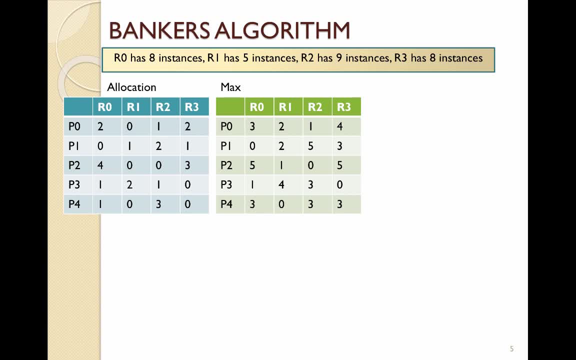 each resource, So P0,, for example. P0 is P0. says indicates that it will need three instances of resource: zero, two instances of one, one instance of two and four instances of three. The operating system will allocate those resources that exist in the system amongst the 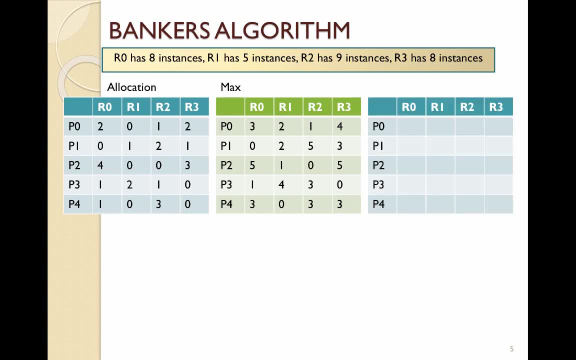 different processes and make decisions on how to allocate these resources in such a way so that we will end up in a safe situation and all processes will be able to complete their work. So, as you can see, the processes have not, the operating system has not allocated all of the resources out and 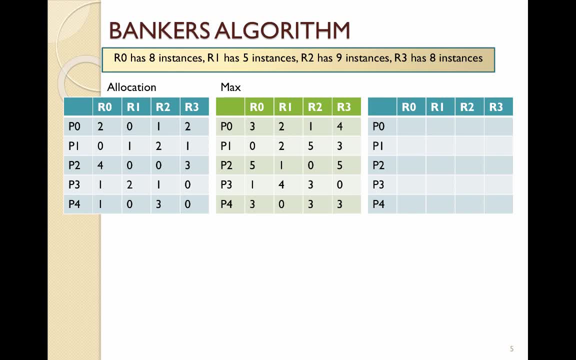 processes have not been allocated the maximum that they need. So to calculate that, to figure that out, you use the Banker's Algorithm, and the Banker's Algorithm has an extra matrix and it also has a. you can see here: it has an extra matrix and it also has a. 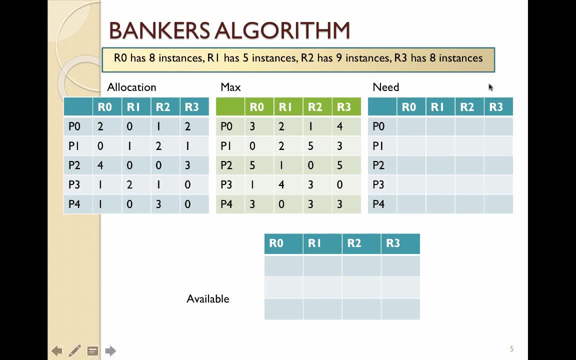 has a vector. So this extra matrix is the need matrix. This need matrix is going to calculate those resources that have been allocated subtracted from the maximum. So, for example, P0 has a maximum of resource zero is three and it has been allocated two, so it needs one more instance of resource zero. And then when? 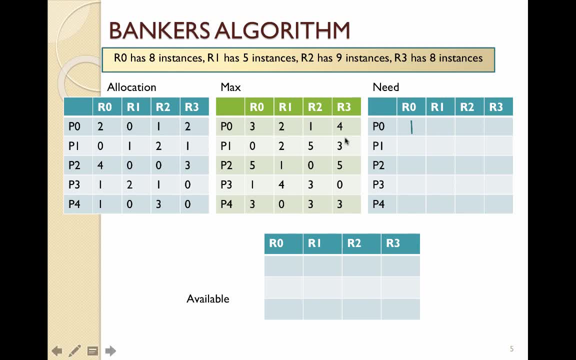 it completes. using that, it will be able to free up for the other processes. And you, and what you do is you calculate the need for all of the process, for all of the resources. So P2 needs two. instance maximum of resource one is two. has been allocated zero, so the need is two. And 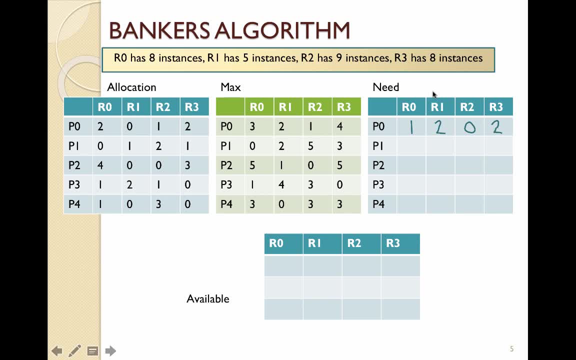 it's just done by simple subtraction and you can get all of the need for all the processes. So I, P1, has a max of zero plus P3 has a maximum of zero plus X1 through 0 and has been allocated 0, a max of 1,. 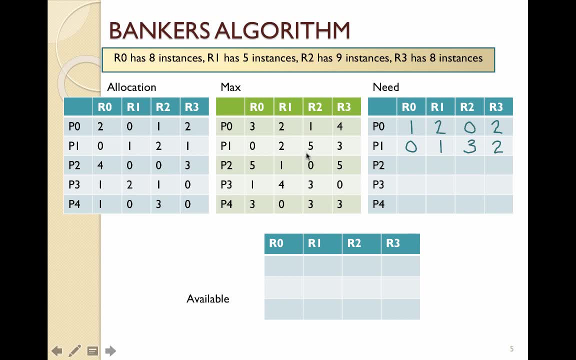 a max of 2 here, and has been allocated 1,, a max of 5 here, and has been allocated 2, and a max of 3 here, and has been allocated 1.. P2 has 5 minus 4,, 1 minus 0,, 0 minus 0,. 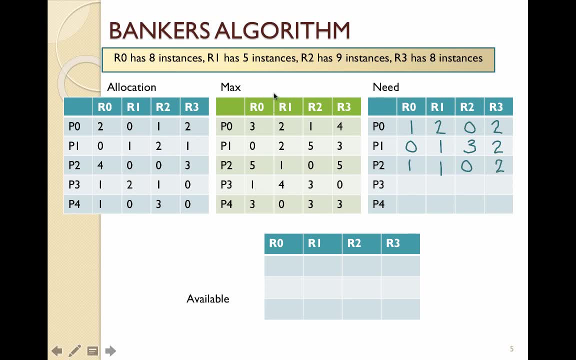 5 minus 3.. P3: 1 minus 1, 4 minus 2, 3 minus 1, 0 minus 0.. P4: 3 minus 2, 0 minus 0,. 3 minus 3 is 0,. 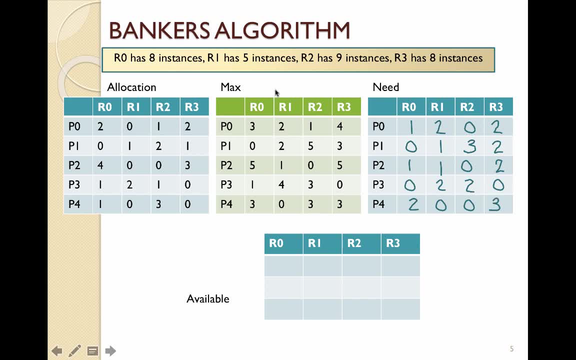 and 3 minus 0 is 3.. So now we've calculated the need and, in order to do the algorithm, what you want to do is you want to see if the available will satisfy the needs of any one process, and then what has been allocated. 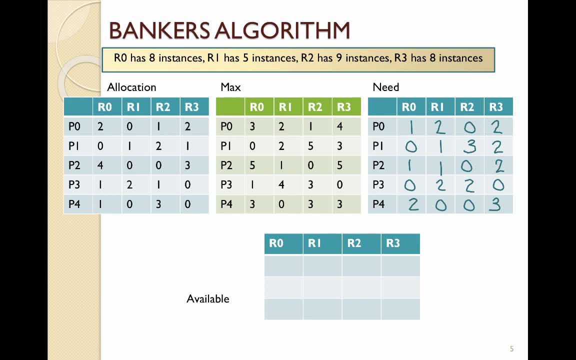 can be freed up for the other processes. So in order to do that, we need to add up what has been allocated for each resource, So resource 0, there are 8 instances of resource 0 that have been allocated at this time and there are 8 that exist in the system, so the available will be 0. 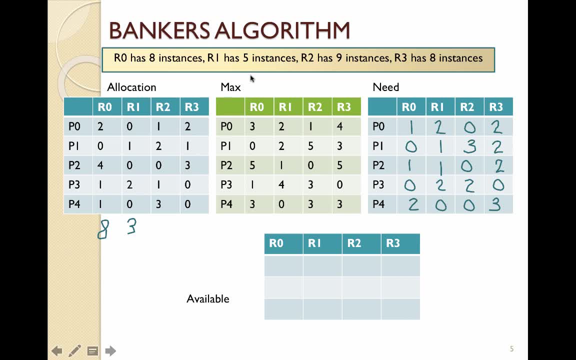 Resource 1, we have 3 that have been allocated and there are 5 in the system, so the available will be 2. and for R2, there are 7 that have been allocated and 9 exist, so the available will be 2. and R3, there are 6 that have been allocated and 8 exist, so the 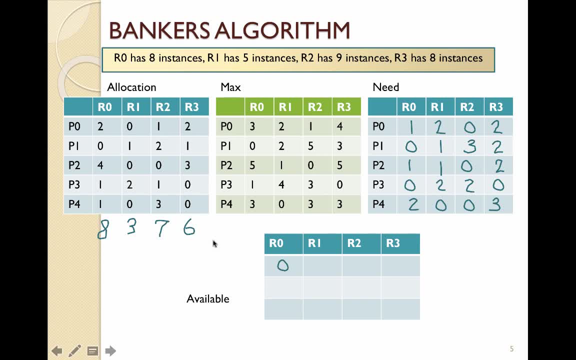 so the available will be 2.. So you can see, here we have 8,. 8 minus 8 is 0,, 5 minus 3 is 2,, 9 minus 7 is 2, and 8 minus 6 is 2.. So now, once we have calculated the need and we have, 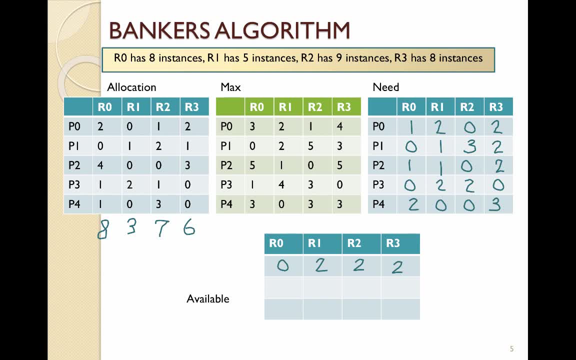 calculated the available, we can go ahead and do the algorithm And to do the algorithm all resources must all available. resources must be greater than the need. So you just go through and you compare the 0, 2, 2, 2. that is available with any process and there's no particular order. 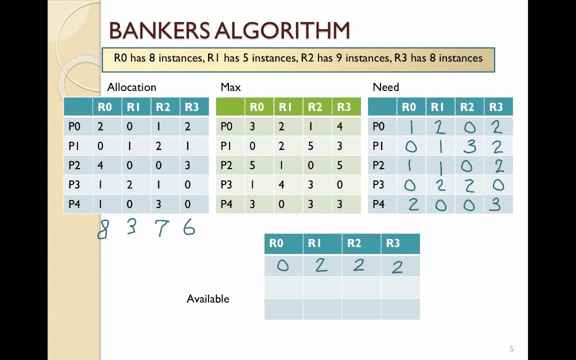 it's just that it has to satisfy the request, the need of the process. So we'll start with P0 and if we have available, 0, 2,, 2, 2. that does not cover the need of P0, but you can see that it does cover the need. 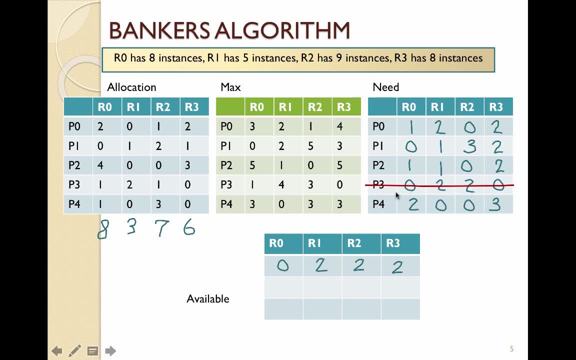 of P3. It doesn't cover P1, P2, but it does cover P3.. 0, 2, 2, 2 is greater than 0, 2, 2, 0.. So what will happen is P3 will be able to. 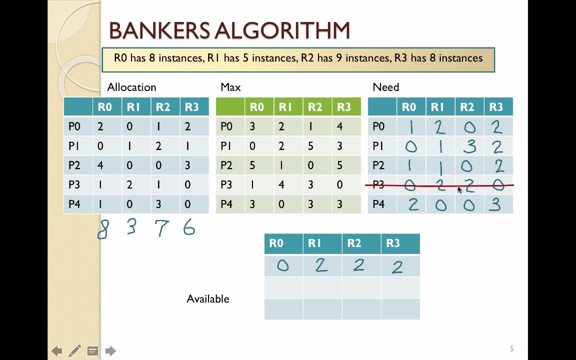 use the resources that are available, finish all, all its work and then those resources that have been allocated to P3 will then become available for the other processes. So this available will note will be put back into the pool of available. this allocated will be put. 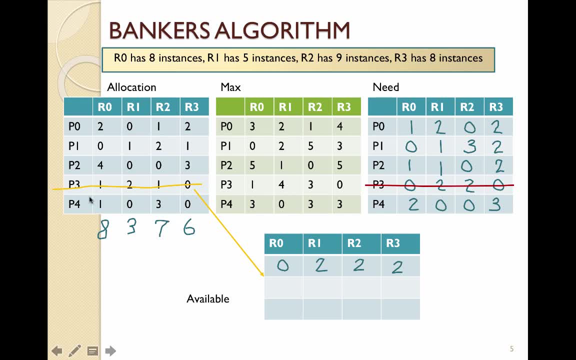 back into the pool of available will be added here. so we will then have: we will take the one two, zero one and add it to the zero two, two, two. so our available will now change to one, four, three, two, and now we take this one, four, three, two. 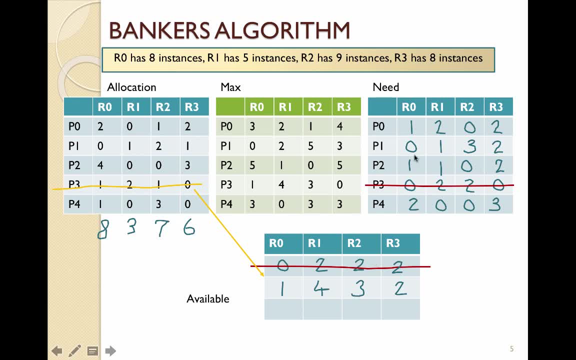 and we go through and we see if we can satisfy the request of any other process, of another process, and you can see that there are a couple we can, so we'll just pick P zero- satisfy the requests of P zero, and then that those that are available, that were allocated to P zero, will then go to available, and so the 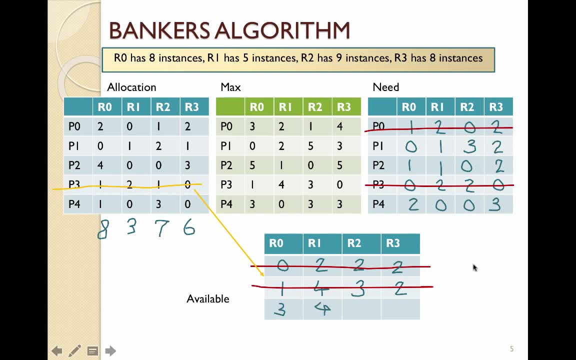 available will then change to 344, for, and the way I got that was by adding the allocation, what has been allocated to P zero to the available, and then P zero is done, and now we have 3, 4, 4, 4, and if you look through you can see that 3, 4, 4, 4 will satisfy the. 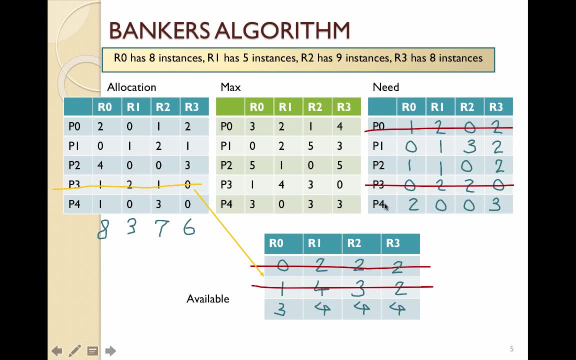 need of any of the leftover processes, so the available can only go up, so we can. so now we know that, yes, this is a safe state, and one sequence for this to be a safe state is p3, p0, p1, p2, p4, and the important part of the sequence is that p3 must be the first one in the sequence, because 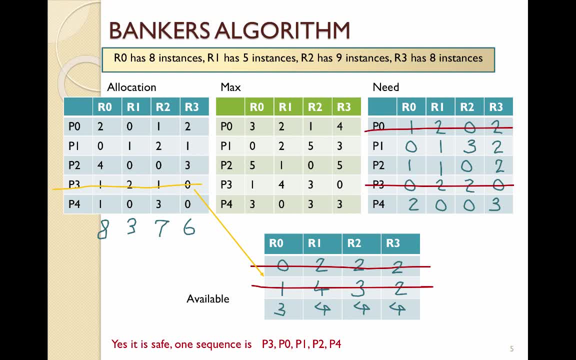 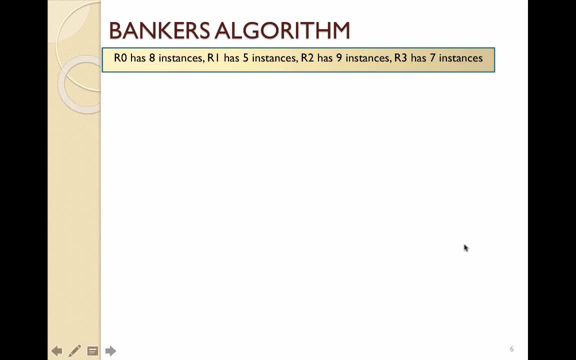 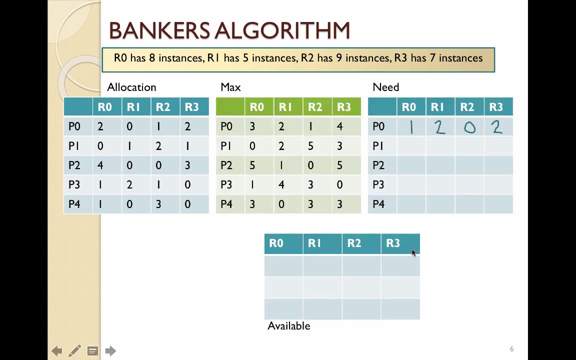 when we initially calculated the available, p3 was the only process that the available could satisfy. so now let's take a quick look at the same situation, only this time r3 does not have eight instances, it has seven instances. so therefore, all of the uh, the need will be. 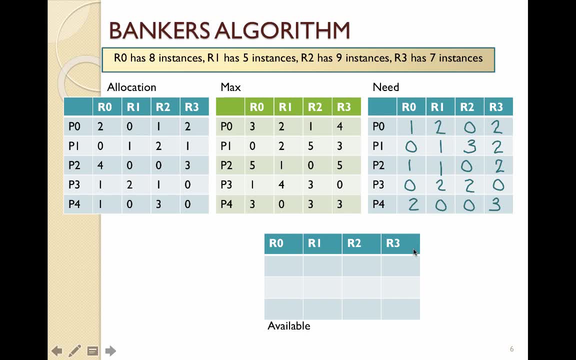 calculated the same and the available will be calculated the same and the available will be calculated the same, calculated differently because, instead of having 8 instances available of R3, we only have 7.. So we will have an available of 0, 2, 2, 1 instead of 0, 2, 2, 2.. 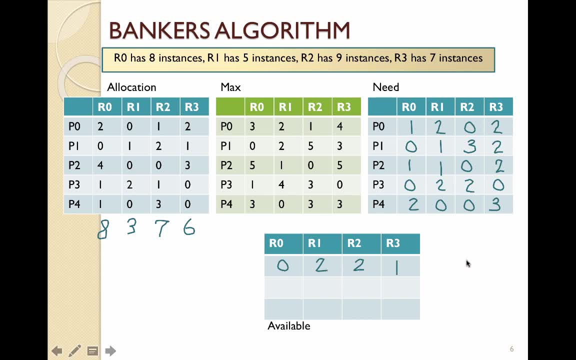 And this is just the example of a situation in which it is an unsafe state. So the only change I made from the last one is that I changed the number of instances that exist for R3.. And so, therefore, when I made this subtraction of 6 that have been allocated from the 7 that 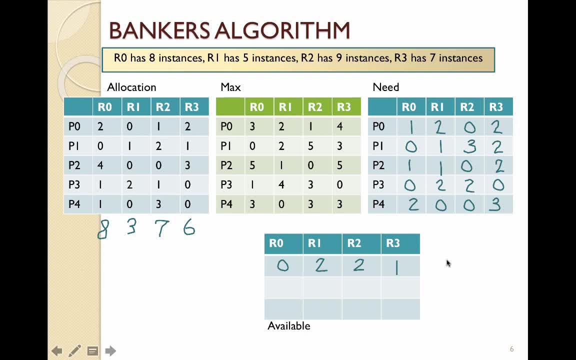 exist, it changed to a 0, 2,, 2, 1.. So now we can proceed through the algorithm and we can see that P3 can be satisfied. So we will take what has been allocated to P3 and add it.